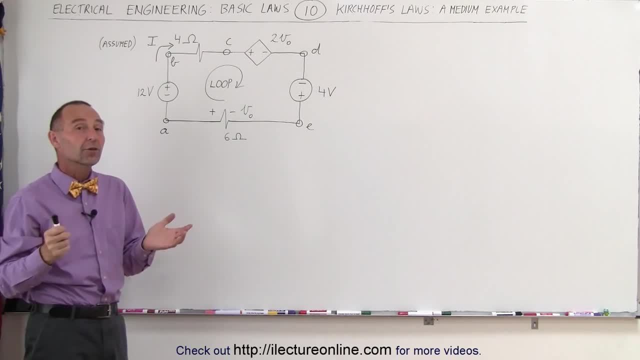 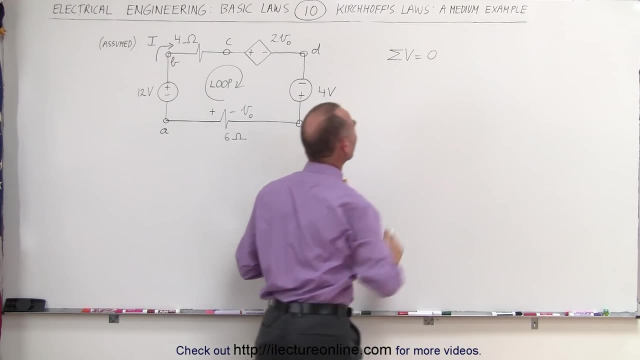 direction. add up all the voltages, Of course, using Kirchhoff's laws, we know that they should add up to zero. We know that the sum of all the voltages around any loop in the circuit must always add up to zero. Let's start at a and go around the circuit. Notice that there are three. 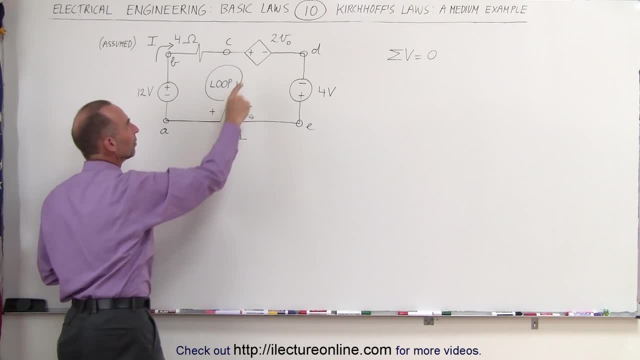 voltage sources. notice there's two resistors. This voltage source is not known, but we know that the voltage across this source is equal to twice the voltage drop across the six-ohm resistor. Also, notice that, even though we're assuming the current is in a clockwise direction, 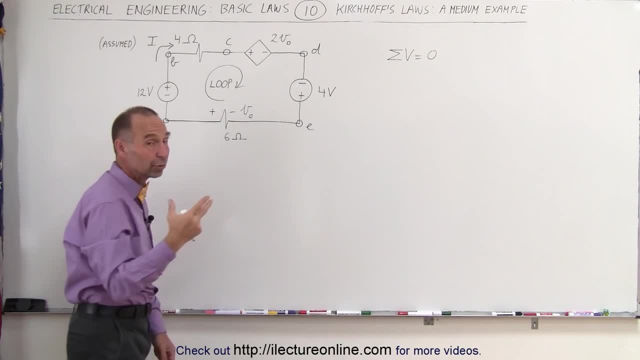 the voltage drop across this resistor would indicate that the actual current is in the opposite direction. But again, that shouldn't really matter. we can change the voltage, We don't have to do that. So I'm going to pick the power after we're done. 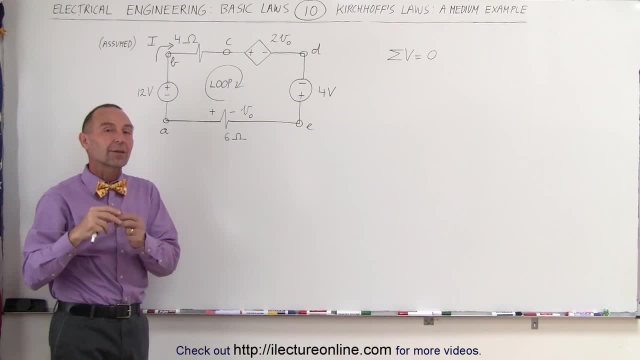 And here we have a circuit that's at the 6-ohm resistor. This circuit has to be at zero. choose the direction any way we like, and if the answer then comes out to be negative, we know that the assumed direction is actually the incorrect direction and the real current is flowing in the 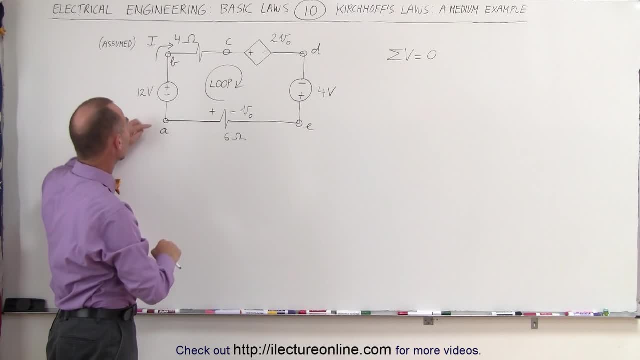 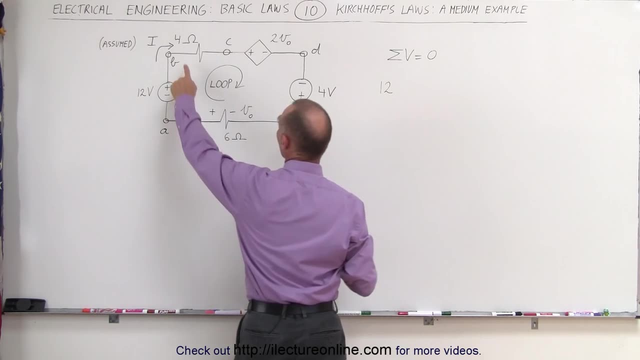 opposite direction. All right, let's go ahead and sum up all the voltages Going from A to B, we cross the 12-volt battery From the negative end to the positive end. that's a 12-volt rise. Now we go. 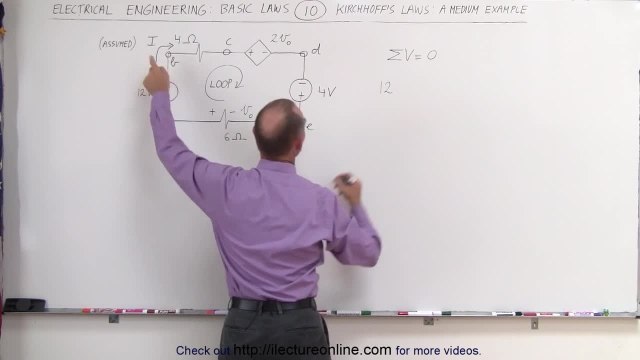 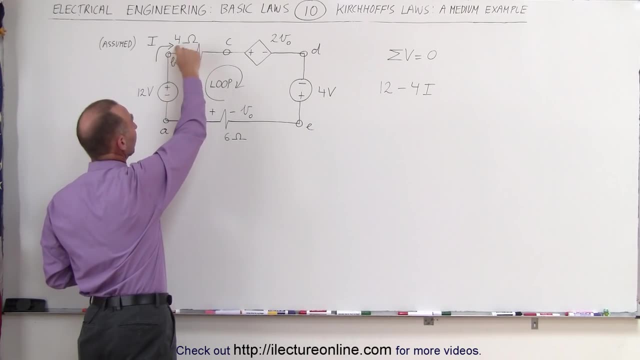 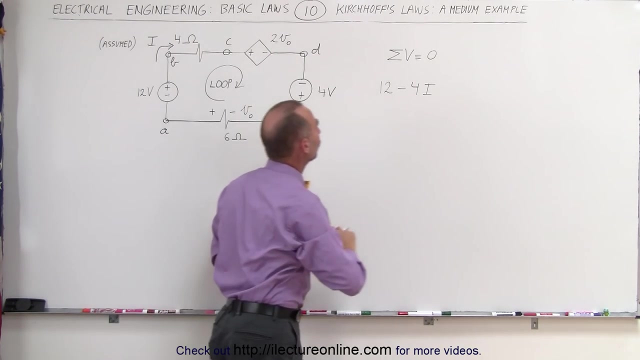 across the resistor Four ohms times the current. that would be a minus four times I voltage drop. Whenever we cross a resistor in the direction of the assumed current, we assume a voltage drop. Here we have a voltage drop across this voltage source equal to minus two V sub naught minus two. 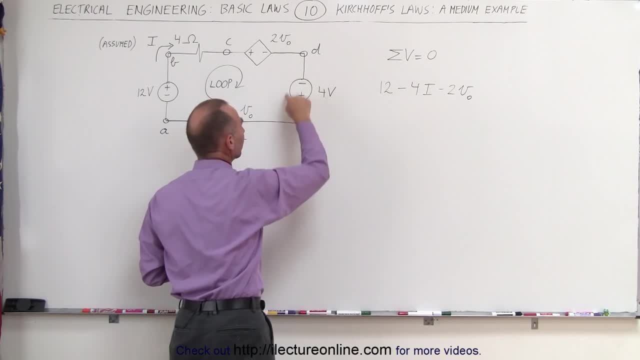 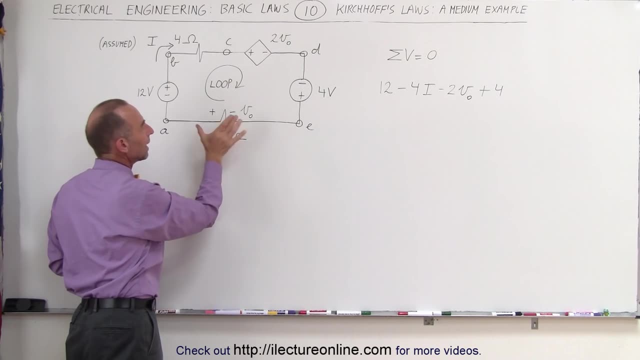 V sub naught. Now we have a voltage rise across this battery or this voltage source. so plus four. and finally, even though we know that the actual voltage drop is from the negative end to the positive end in this direction, we're just going to assume the direction. the current is clockwise. 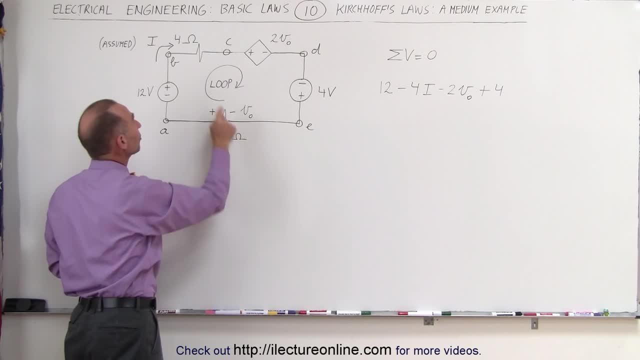 and there's a voltage drop. Now let's go ahead and sum up all the voltages From the negative end to the positive end. therefore, we assume a voltage drop six ohms times the current, minus six times the current, and that 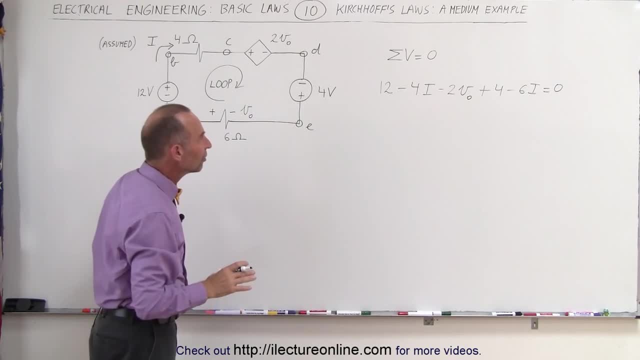 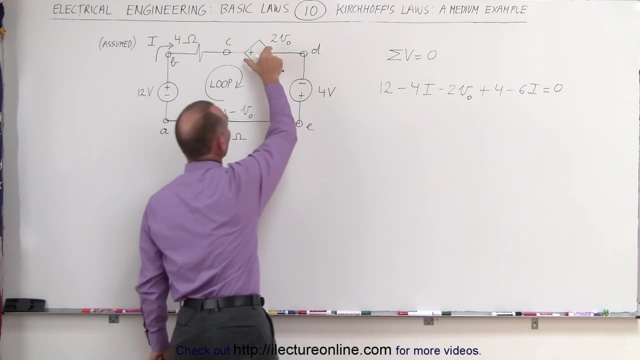 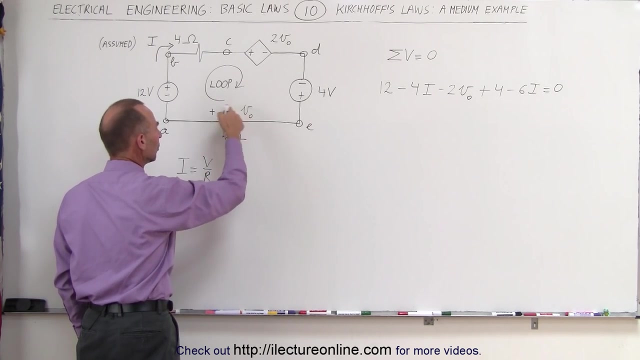 adds up to zero, A second equation that we can use to solve the problem, because what we're trying to do here is solve for the current in the circuit and solve for the voltage across this voltage source. We're going to use Ohm's law- I equals V over R- to determine a relationship between the 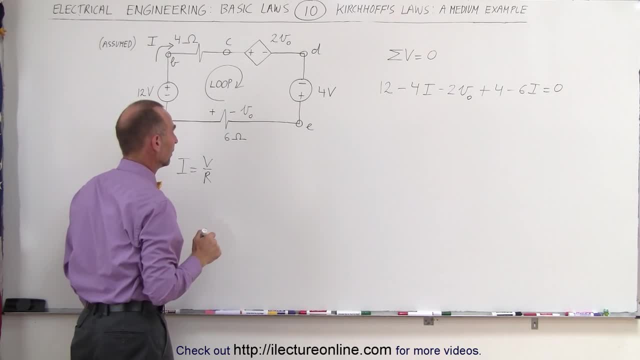 current and V sub naught, using what's happening on this resistor. Here we can see that the voltage drop across this resistor is V sub naught, but since we assume the current to be in this direction, that would cause this to be a voltage drop, and since it actually 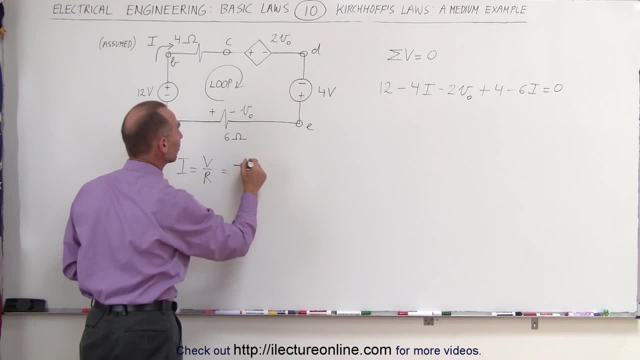 looks like it's a voltage rise. this, therefore, is equal to minus six V sub. naught, That's the voltage drop across the resistor. It's, in essence, a voltage rise divided by the resistance. Oh, I'll Hold it, hold it. hold it Back up. So this is equal to the voltage across that. It is going to be a minus V sub. 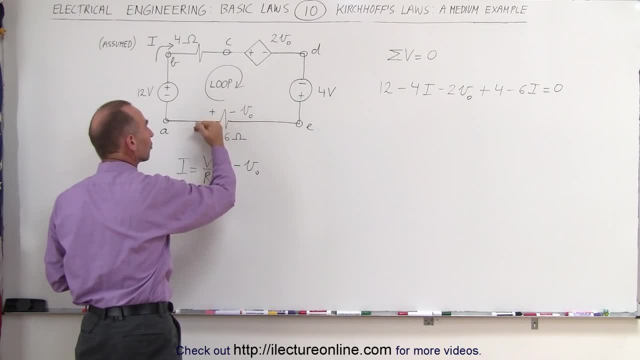 naught. Why minus? Because we're assuming the current to be in this direction, which causes, which should make this a voltage drop, but instead it's a voltage rise. so we have to put a minus in there, divided by the resistance, which is six ohms, Solving this for V sub naught. we can then see that V sub naught across the. 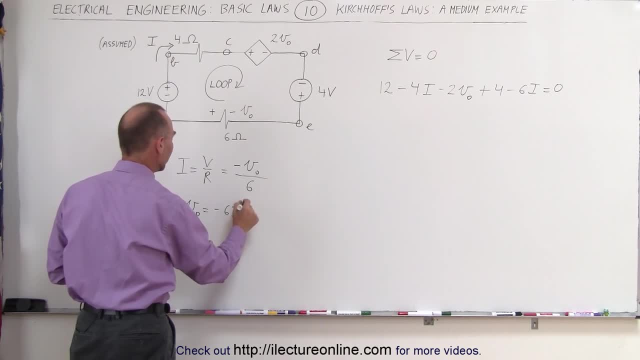 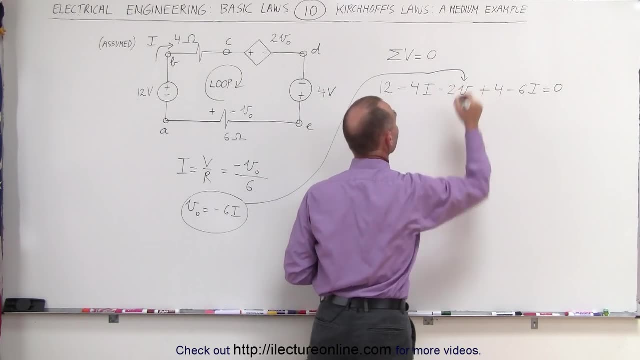 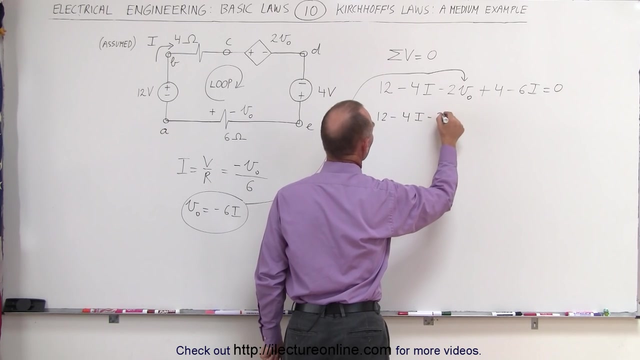 resistor is equal to minus six ohms, equal to minus six times I, which we then substitute into our equation here. so we need to plug that right in there. That allows us to solve for the current 12 minus four times I minus two times V. 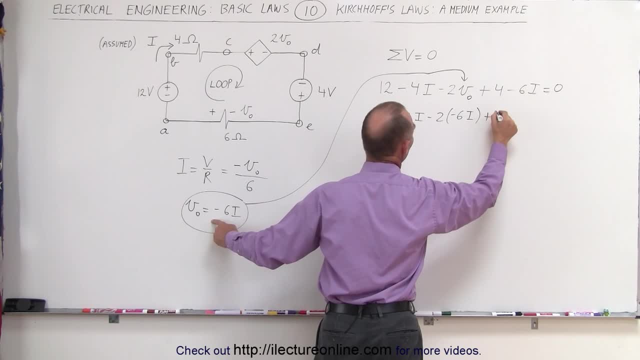 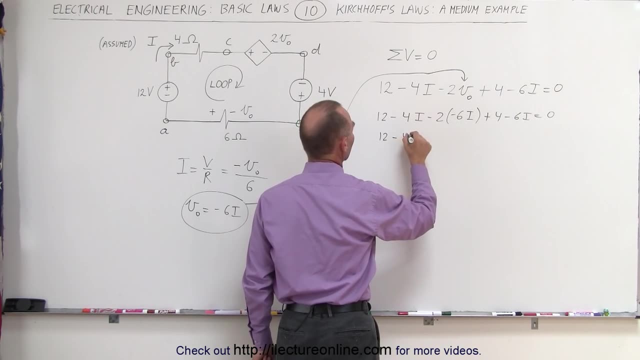 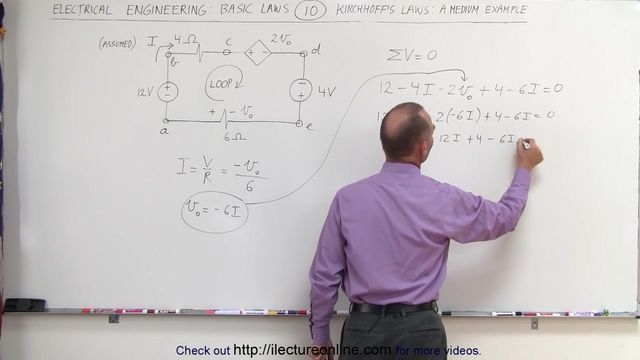 sub naught, which is a minus six. I plus four minus six, I is equal to zero. Let's go ahead and get rid of that. So we have. we have a minus V sub naught plus 12. I plus four minus six, I is equal to zero. 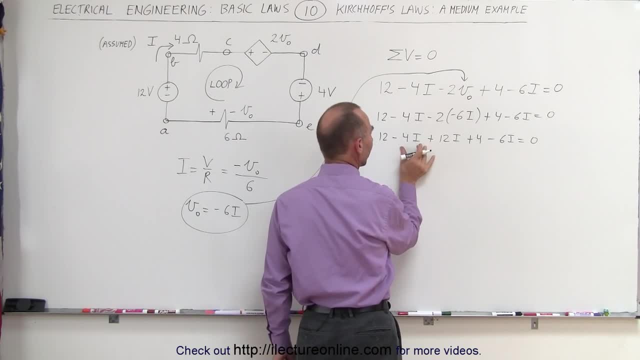 adding up all the currents on the left side- minus four, plus 12, minus six, that is two I- and moving all the voltages or the numbers to the other side, that becomes a minus 12 and a minus four or two I. 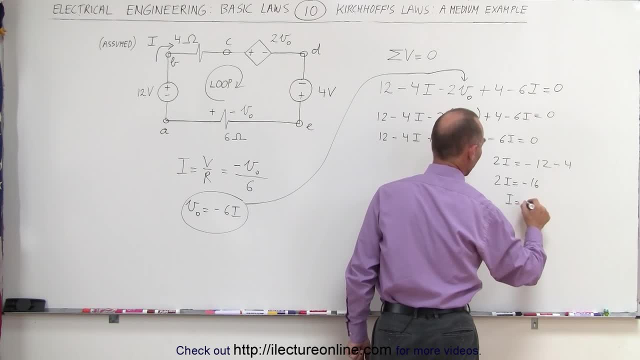 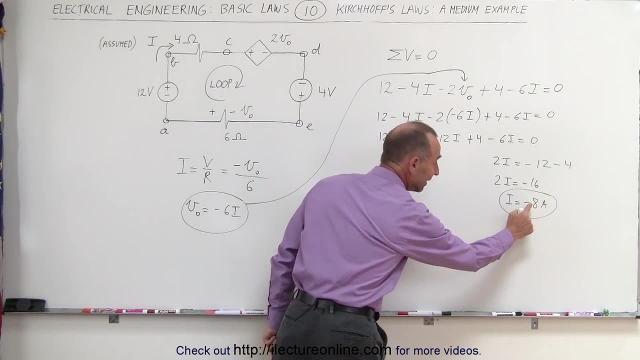 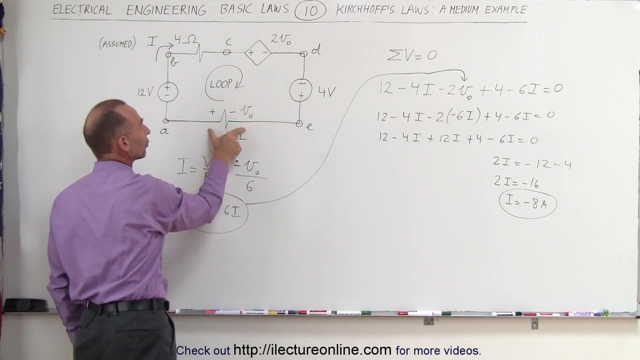 is equal to minus 16, or I is equal to minus eight amps divided on both sides by a two. Now we know that we have a negative voltage drop in the circuit and notice the sign a negative eight amps. We assumed that that would be the case, that we would have a real current in the opposite.